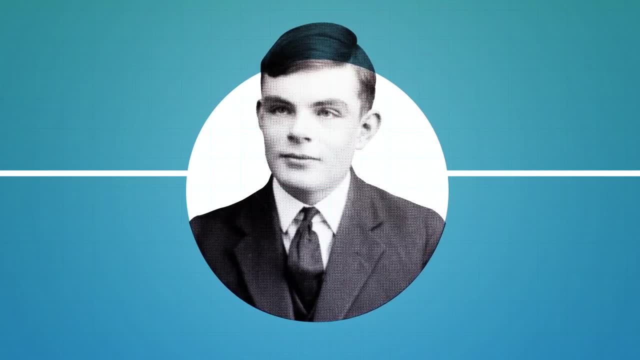 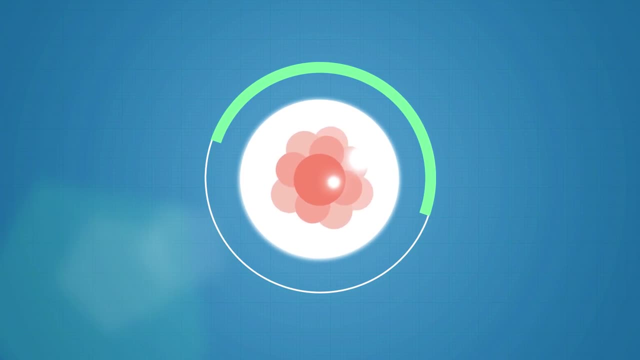 during his short lifetime, Alan Turing also proposed a theory to help explain a series of patterns that recur over and over again throughout the natural world, like the spherical organization of cells in an embryo, the spiral arrangement of petals on a flower, the world's 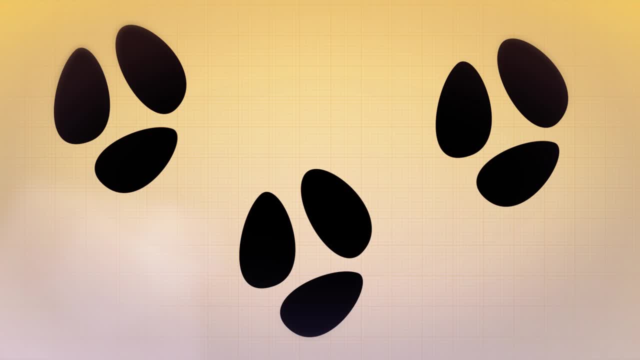 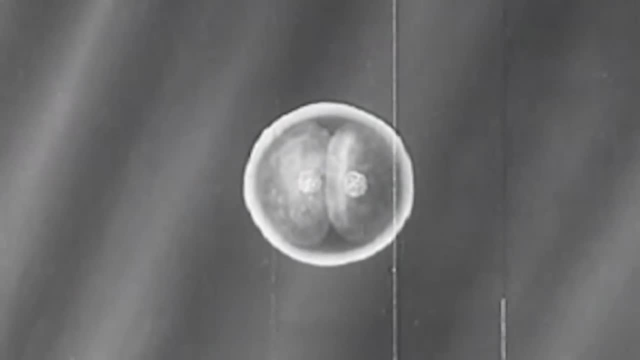 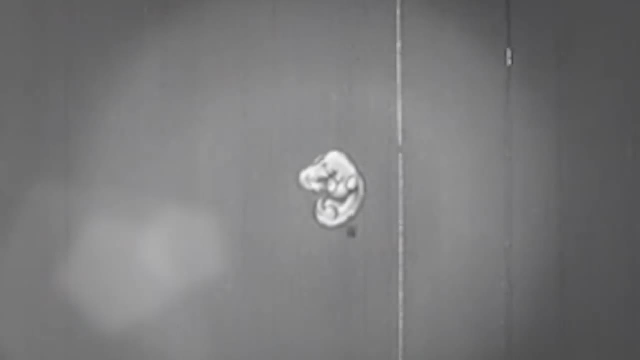 tentacle pattern of a hydra, the waves on a sand dune, the spots on a leopard and even the stripes on a zebra. Turing's desire to understand nature's reoccurring patterns stemmed from his fascination with embryology. Turing wanted to know how the small, uniform ball of cells in an embryo could. 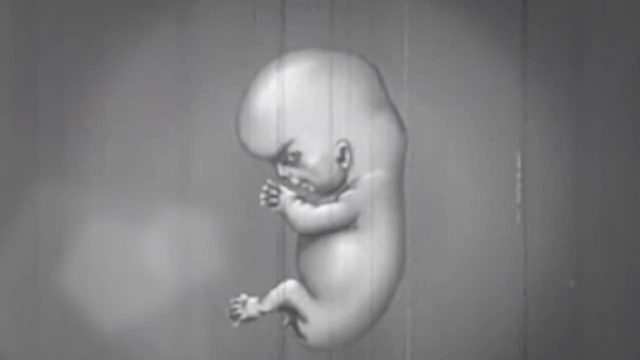 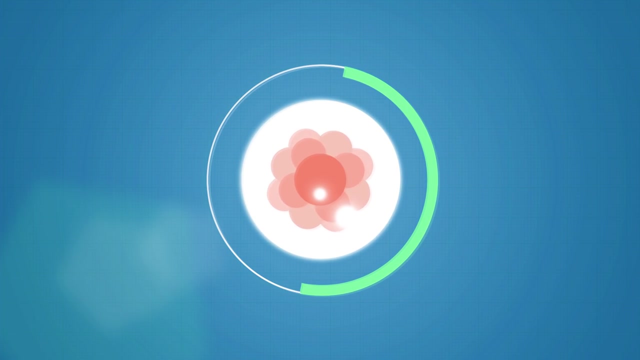 differentiate and morph into a fully formed complex being. His hunch was that there had to be some mathematical principle underpinning the reoccurring patterns in an embryo's development. So in 1952, Turing published a paper called The Chemical Basis of Morphogenesis. 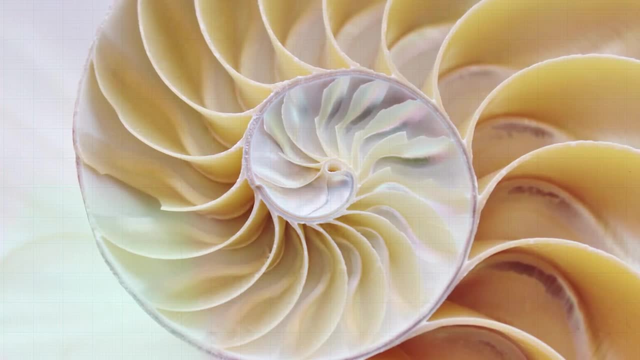 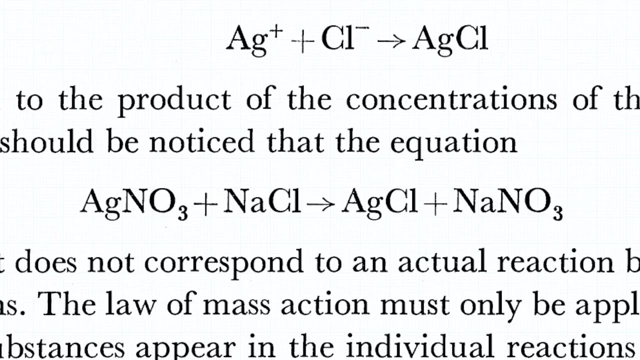 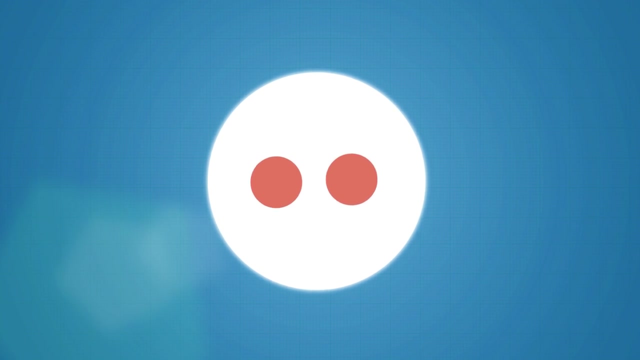 Within it he proposed that the diversity of patterns we see in nature can be explained by a mathematical model called the reaction-diffusion system. While the entire model is too complex to explain here, essentially the system can be broken down like this. Let's say we have two identical cells within an embryo. In the mix are two. 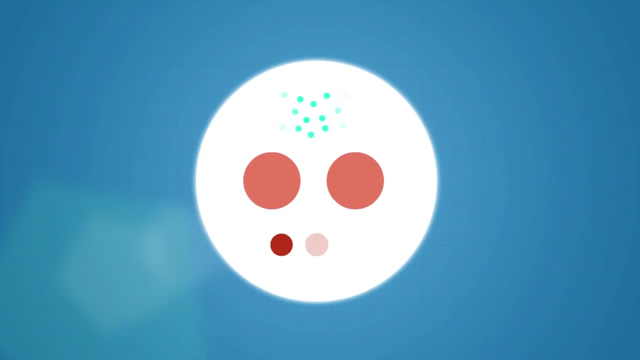 chemicals that can either activate or inhibit a specific reaction within an embryo's cells Turing called these morphogens. As these morphogens diffuse through the embryo, they cause the cells around them to transform, ultimately creating patterns like spots, stripes, spirals, hexagons and whirls. But this is just one example of the reaction-diffusion. 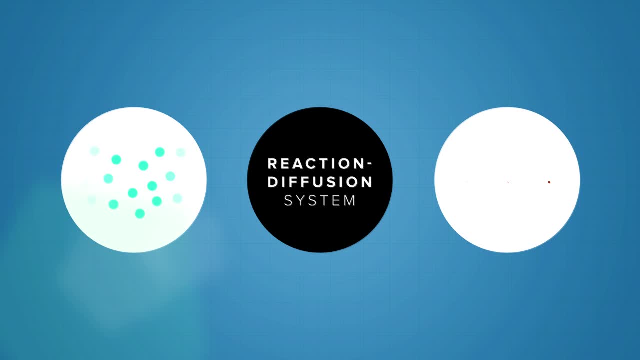 system at work. Morphogens can really be any two chemical substances that work together to stop and start a reaction, like hormones, proteins or acids, And changing the rate at which these components interact. diffuse and decay determines the rate at which these compounds can interact. 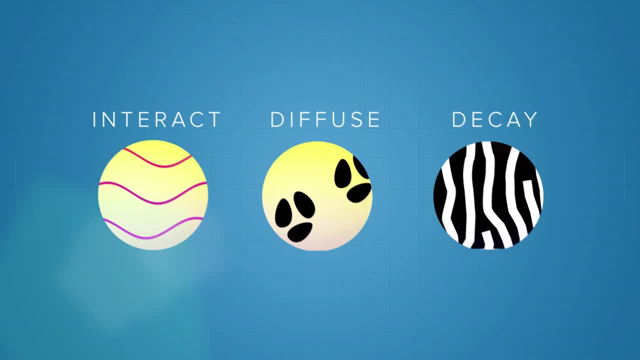 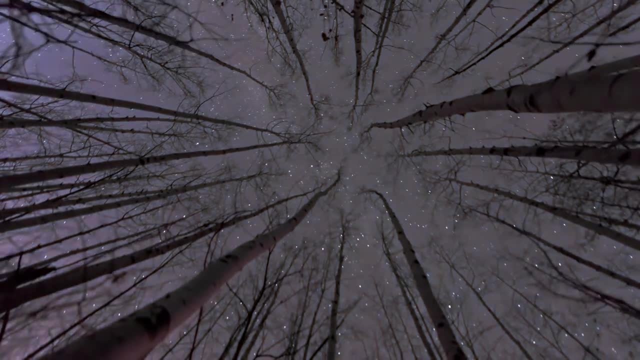 determines the way those elemental patterns like waves, spots and stripes appear. Today, many theoretical biologists and mathematicians believe that Turing's system could also be applied to the patterns found in vegetation on a landscape, weather systems and even to the formation of galaxies. 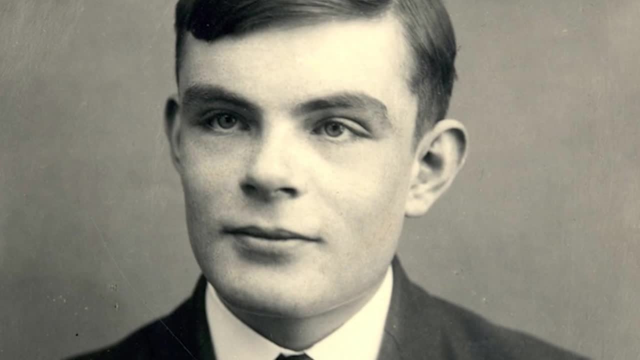 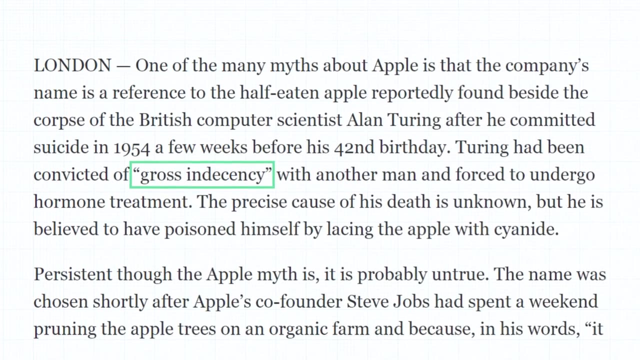 Sadly, Turing never found out whether his theory was right. In an age of intolerance, he took his own life in 1954 following a conviction for gross indecency, the charge for being openly gay, And for a long time afterward his ambitious model was forgotten.